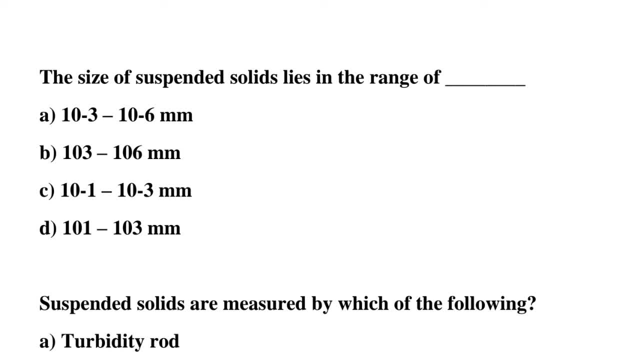 Option A: 10 power minus 3 to 10 power minus 6 mm. Option B: 10 power- 3 to 10 power- 6 mm. Option C: 10 power minus 1 to 10 power minus 3 mm. Option D: 10 power 1 to 10 power- 3 mm. 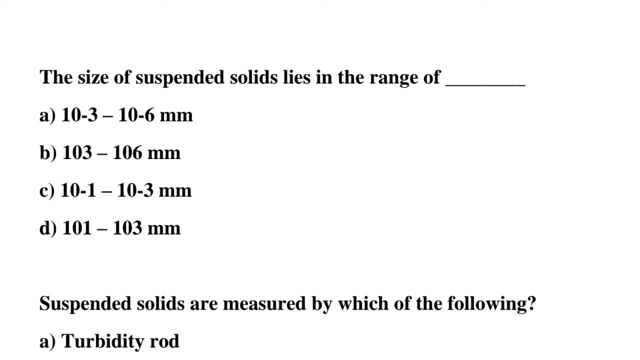 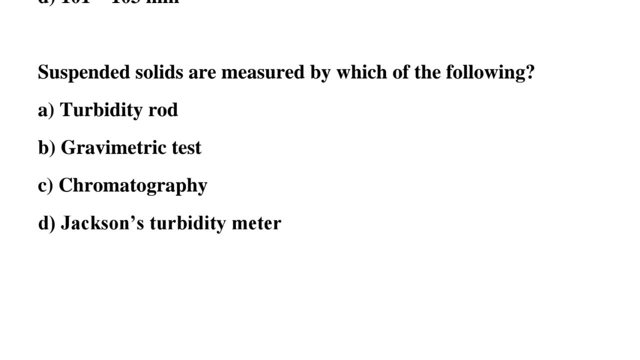 So the correct answer is option C: 10 power minus 1 to 10. power minus 3 mm. So next question: suspended solids are measured by which of the following? Option A- turbidity dot. Option B- gravimetric meter. 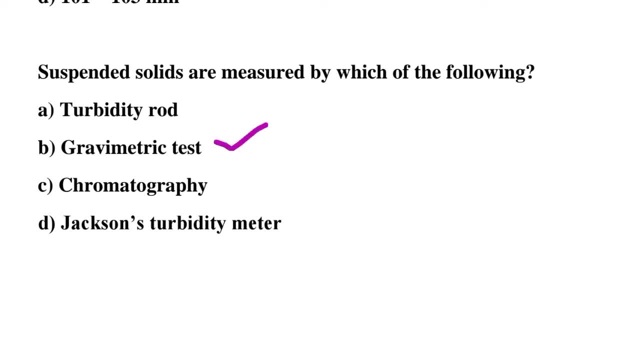 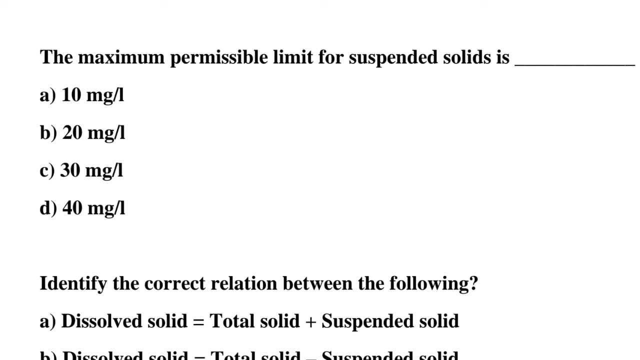 Option C, chromatography. Option D, jacks and turbidity meter. So the correct answer is option B, gravimetric meter. So next question: the maximum permissible limit for suspended solids is Option A, 10 milligram per liter. Option B, 20 milligram per liter. 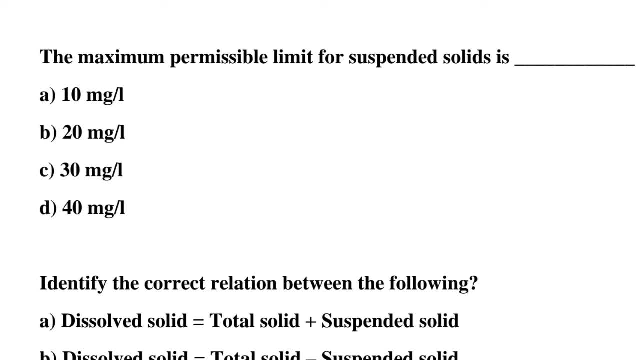 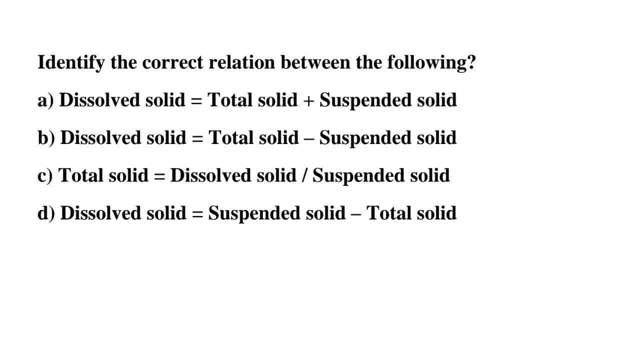 Option C, 30 milligram per liter. Option D: 40 milligram per liter. So the correct answer is option C, 30 milligram per liter. So next question: identify the correct relation between the following: Option A- dissolved solids. 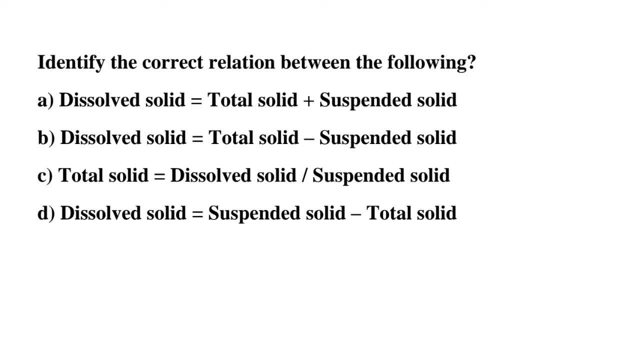 Option B, dissolved solids. Option C, dissolved solids. Option D, dissolved solids. So the correct answer is option B, dissolved solids. So next question: which of the methods is used to measure the color of water? Option A, gravimetric analysis. 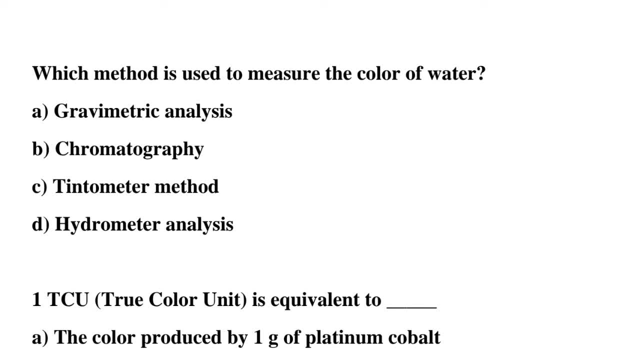 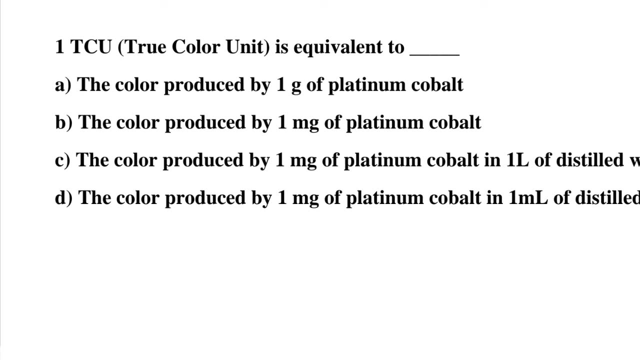 Option B- chromatography. Option B- Chromatography. Option C- Tintometer. Option D- Hydrometer analysis. So the correct answer is option C, Tintometer method. So next question 1, TCU. that is true, color unit is equivalent to option A. 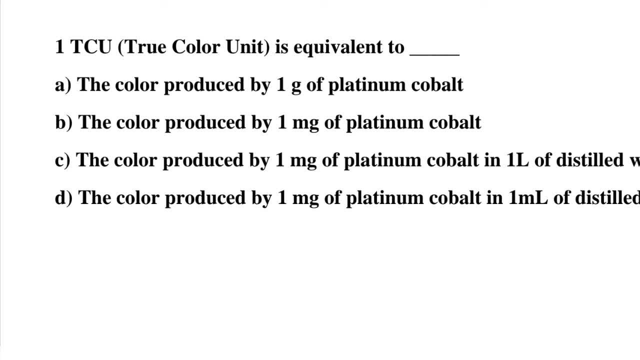 The color produced by 1 gram of platinum cobalt- Option B. The color produced by 1 milligram of platinum cobalt- Option C. The color produced by 1 milligram of platinum cobalt in 1 liter of distilled water. 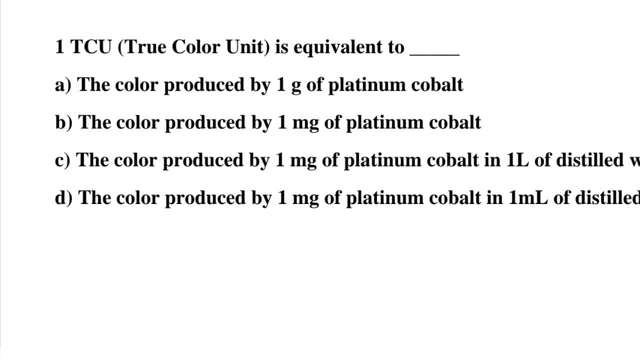 Option D: The color produced by 1 milligram platinum cobalt in 1 ml of distilled water. So the correct answer is option C: The color produced by 1 milligram of platinum cobalt in 1 liter of distilled water. So next question. 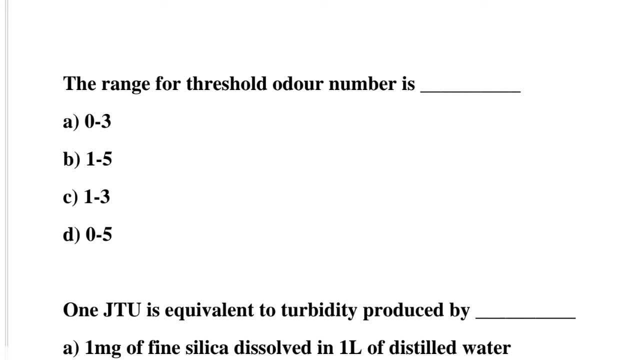 The range for the threshold order in number is option A: 0 to 3.. Option B: 1 to 5.. Option C: 1 to 3.. Option D: 0 to 5.. So the correct answer is option C: 1 to 3.. 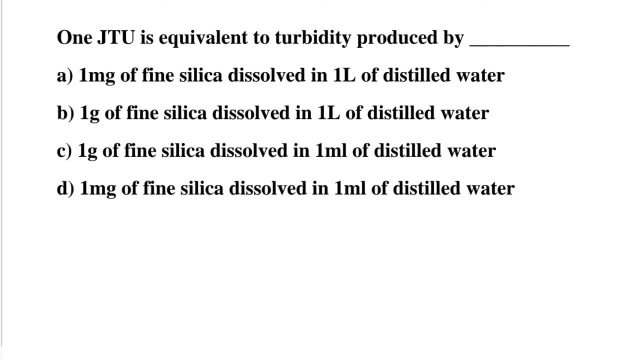 So next question: 1 JTU is equivalent to turbidity produced by: option A: 1 milligram of fine silica dissolved in 1 liter of distilled water. Option B: 1 gram of fine silica dissolved in 1 liter of distilled water. 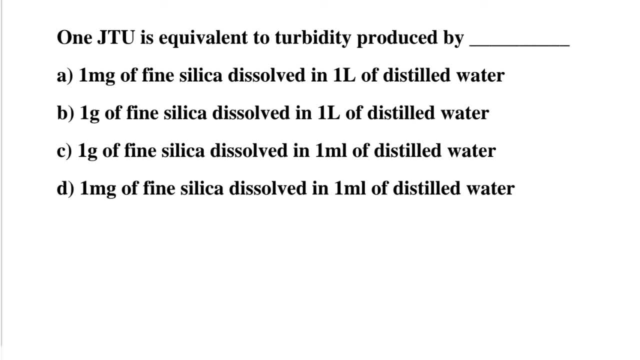 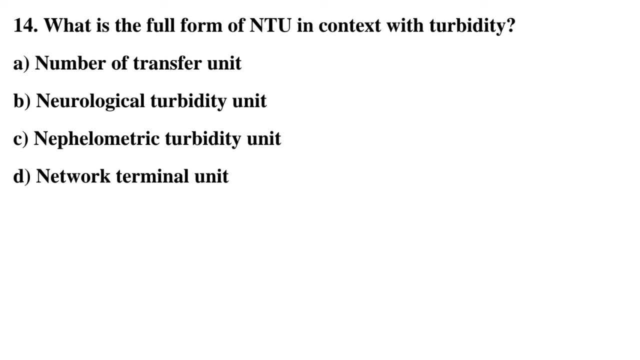 So the correct answer is option C: 1 gram of fine silica dissolved in 1 ml of distilled water. What is the full form of NTU in contact with the Turbidity? A? Number of transfer unit. B- Neurological turbidity unit. 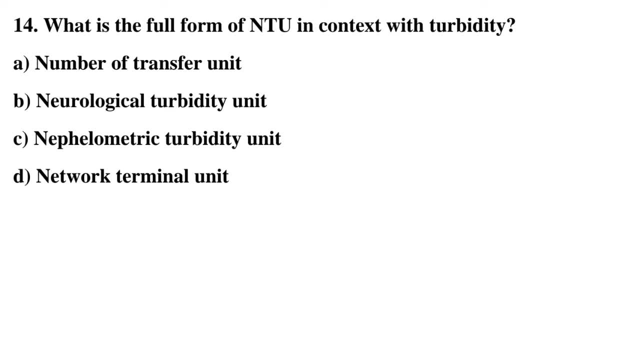 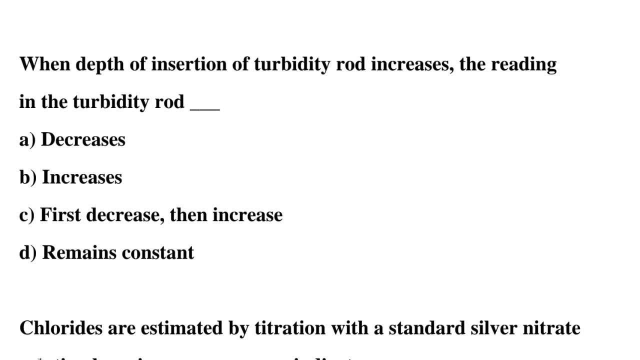 C- Nephrologic turbidity unit. D- Network terminal unit. So the correct answer is option C- Nephrologic turbidity unit. So the correct answer is option C- Nephrologic turbidity unit. Next question: When depth of insertion of the turbidity rod increases, the reading in the turbidity rod? 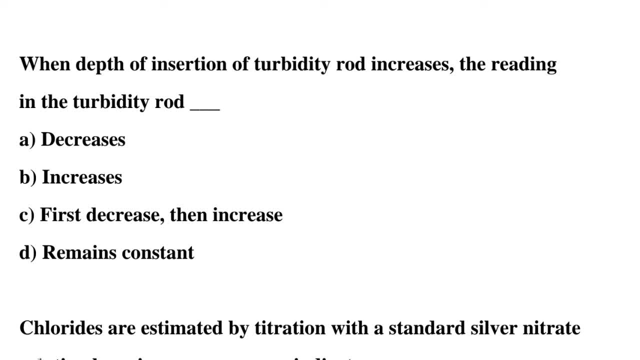 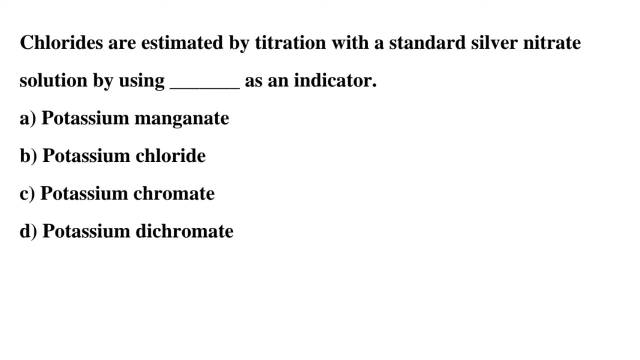 Option A Decreases. Option B Increases. Option C First decreases, then increases. option D remains constant. so the correct answer is option A decreases. so next question: chlorides are estimated by titration with the standard silver nitrate solution by using dash as indicator. option A: potassium magnet. option B: potassium chloride. option C: potassium chromate. 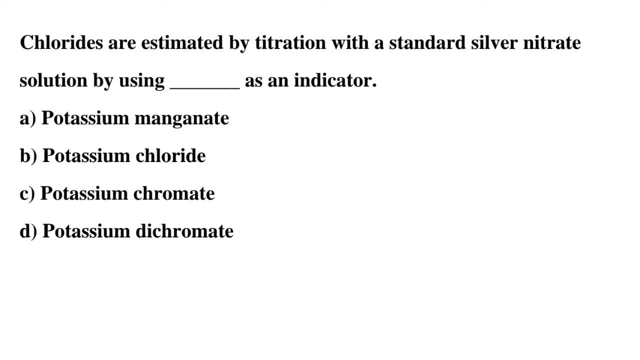 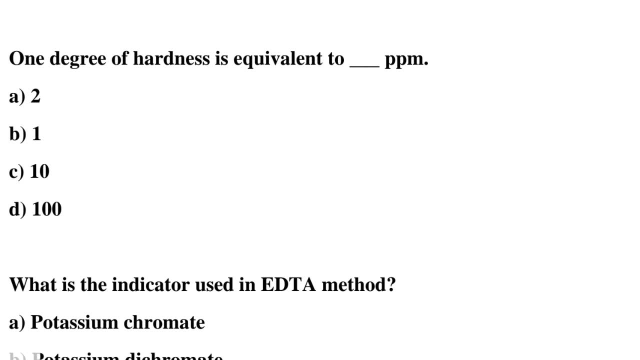 option D- potassium dichromate. so the correct answer is option C, potassium chromate. so next question: one degree of hardness is equivalent to dash ppm. option A 2. option B 1. option C: 10 option D: 100. so the correct answer is option B 1. so next question: what is the indicator used in? 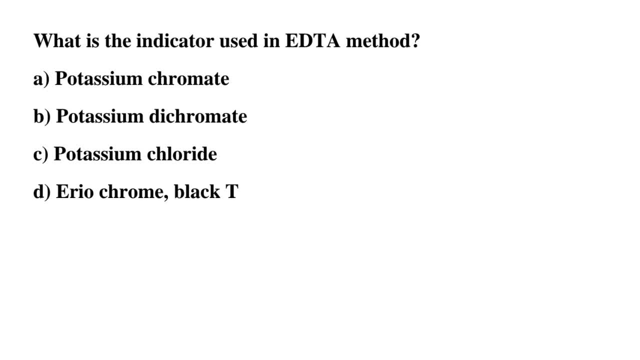 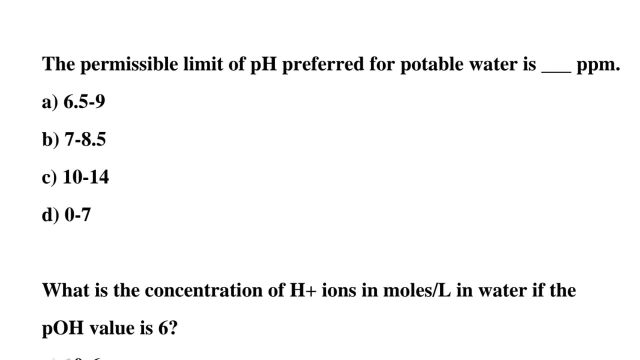 EDTA method. option A- potassium chromate. option B- potassium dichromate. option C- potassium chloride. option D- areochrome black tea. so the correct answer is option D- areochrome black tea. so next question: the permissible limit of pH preferred for portable water is dash ppm. option A is 6.5 to 9 ppm. 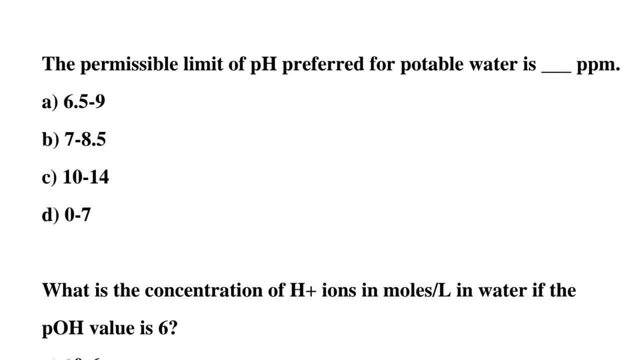 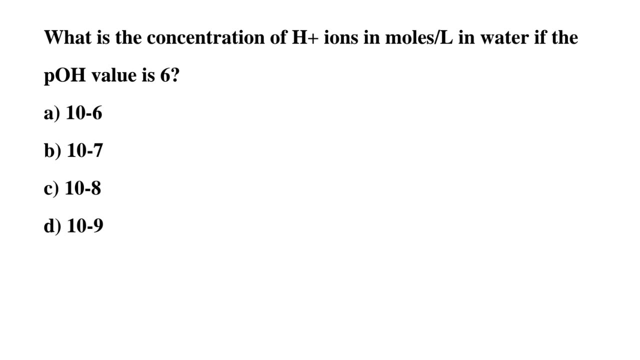 option B, 7 to 8.5 ppm. option C, 10 to 14 ppm. option D: 0 to 7 ppm. so the correct answer is option A, 6.5 to 9 ppm. so next question: what is the concentration of H plus ions in moles by liter in water if the 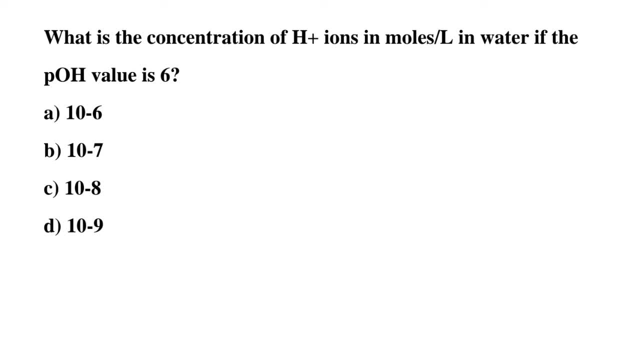 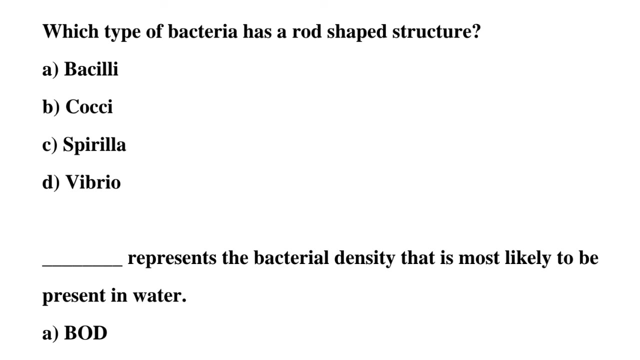 value is 6. option A: 10 power minus 6. option B: 10 power minus 7. option C: 10 power minus 8. option D: 10 power minus 9. so the correct answer is option C: 10 power minus 8. so next question: which type of bacteria has a rod shaped structure? 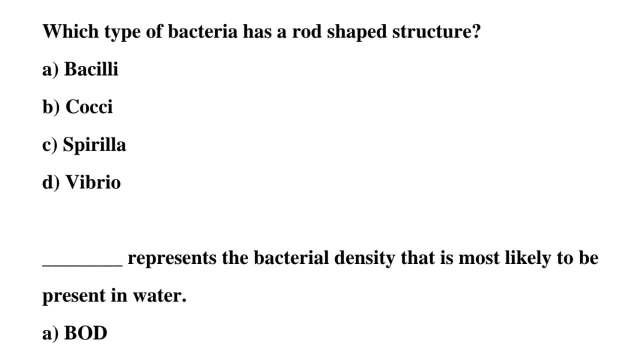 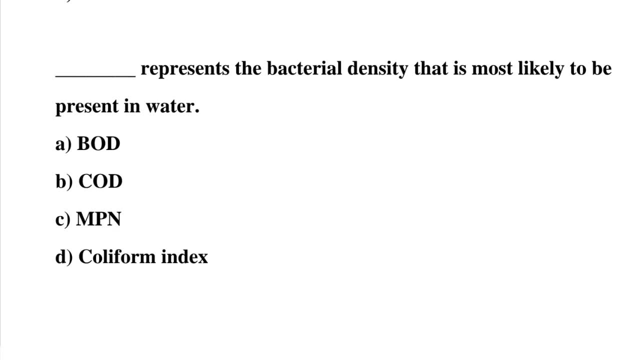 option of a. basic. option B: cookie absence. the absence e spirula. option D: vibrio. so the correct answer is option a, basically. next question: that represents a bacterial density that is most likely to be present in water, option 8 ppm. so, anyhow, all the solutions are also. 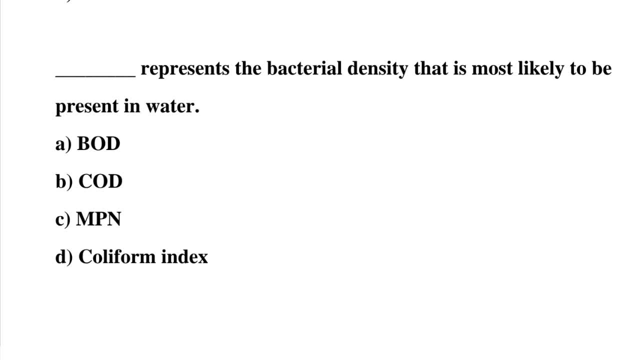 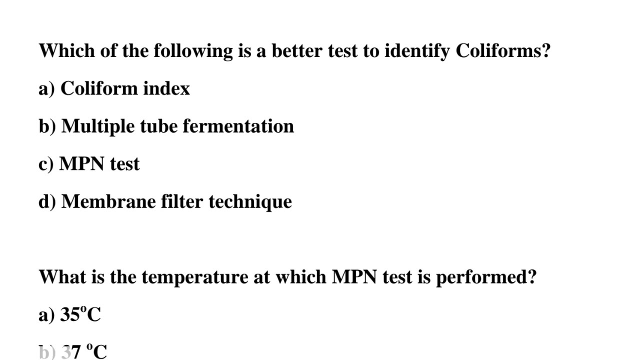 in bod. option b- cod. option c- mpn. option d- coliform index. so the correct answer is option c- mpn. which of the following is better taste to identify the coliforms? option a- coliform index. option b- multiple tube fermentation. option c- mpn test. option d- membrane filter technique. so the correct 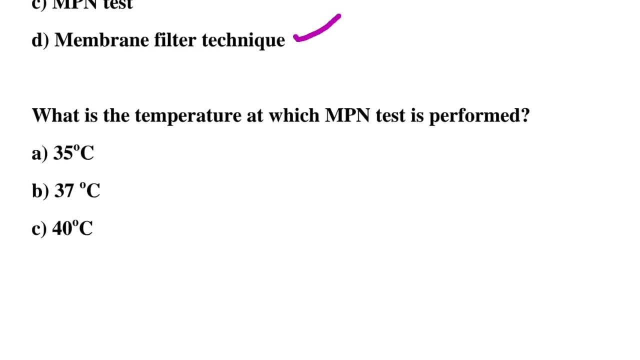 answer is option d, membrane filter technique. next question: what is the temperature at which mpn test is performed? option a: 35 degree celsius. option b is 37 degree celsius. option c, 40 degree celsius. option d: 45 degree celsius. so the correct answer is option b, 37 degree celsius. so next: 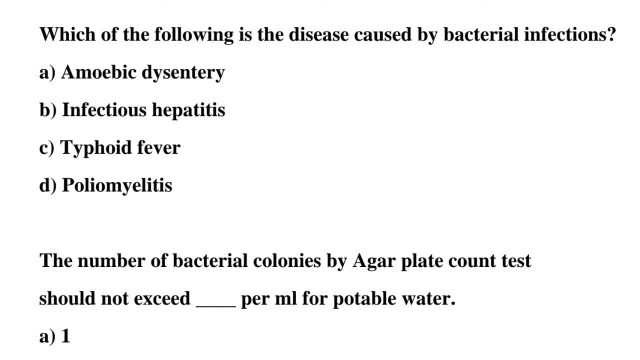 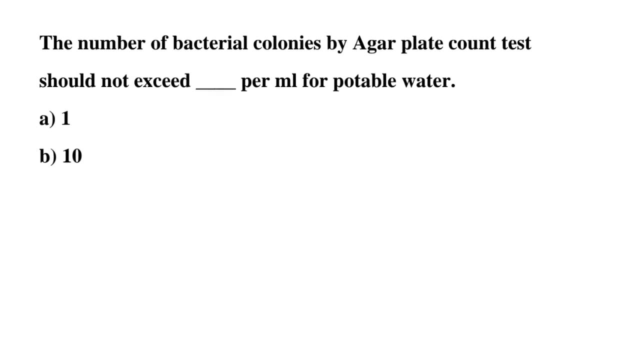 question: which of the following is the disease caused by bacterial infections? option a- amoebic dysentery. option b- infectious hepatitis. option c- typhoid fever. option d- polymyelitis. so the correct answer is option c, typhoid fever. so next question: the number of bacterial colonies by auger plate count test should not.